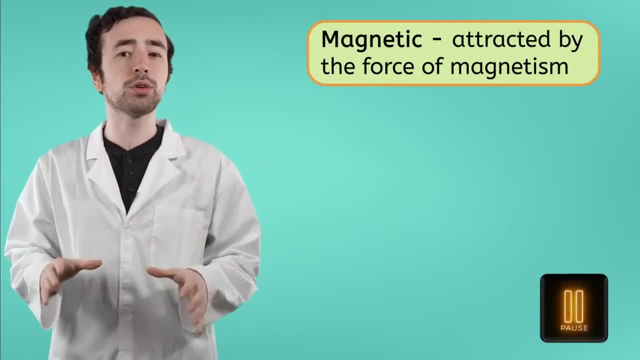 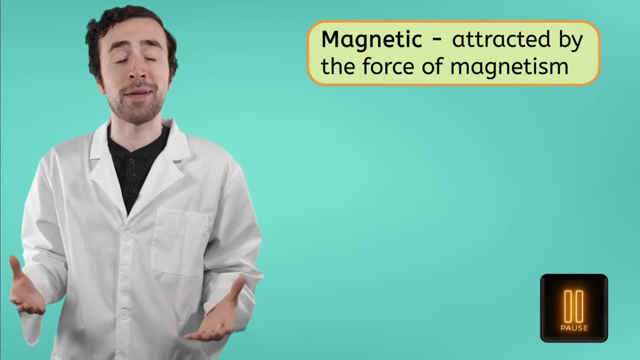 If you have a magnet lying around your house right now, pause the video here to investigate what types of materials are magnetic. If you don't have a magnet lying around, that's totally fine too. Just think about any past experiences and observations you might have Either way. 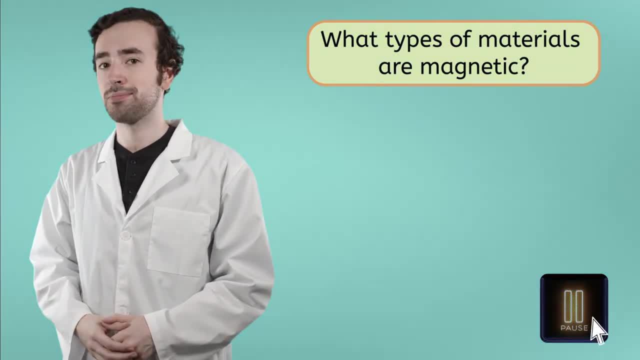 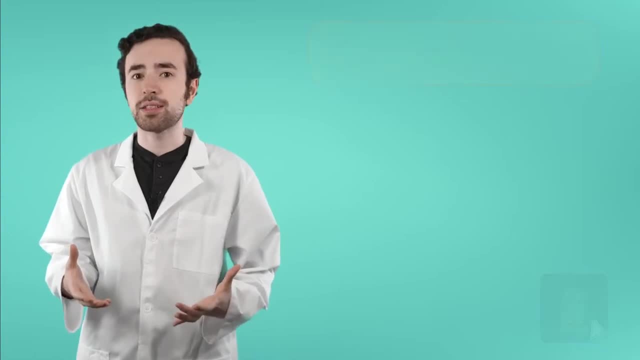 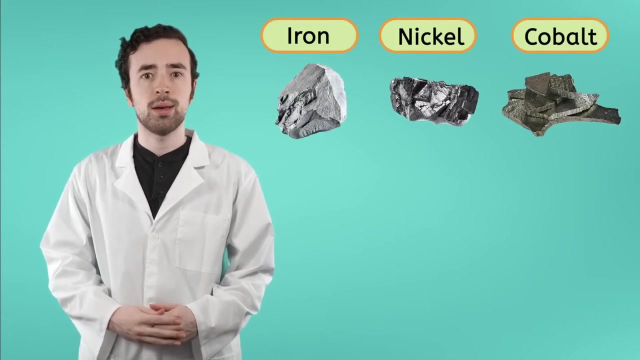 jot down your thoughts in your guided notes. now You probably noticed that most of the things that stick to magnets are metal. As a matter of fact, the most magnetic materials out there are the metals iron, nickel and cobalt. However, just because something is a metal, it doesn't mean it's magnetic. 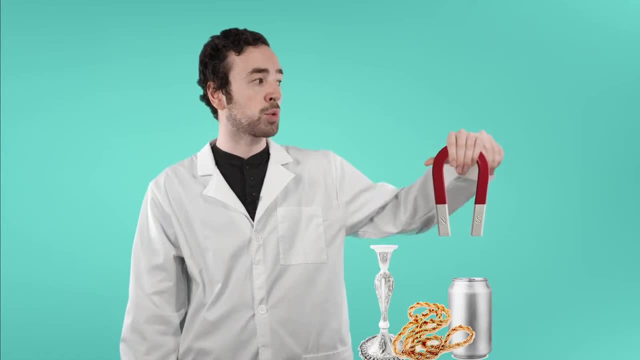 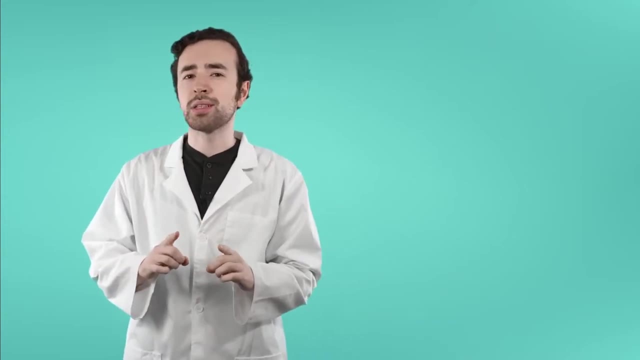 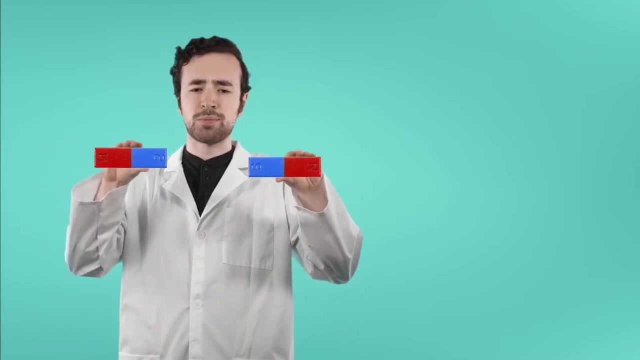 If you try to move a magnet over some silver, gold or aluminum, then you might as well be holding a rubber chicken for all you're going to attract. You might have also noticed that magnets don't always attract things. Sometimes when you take two different magnets and try to push them together, 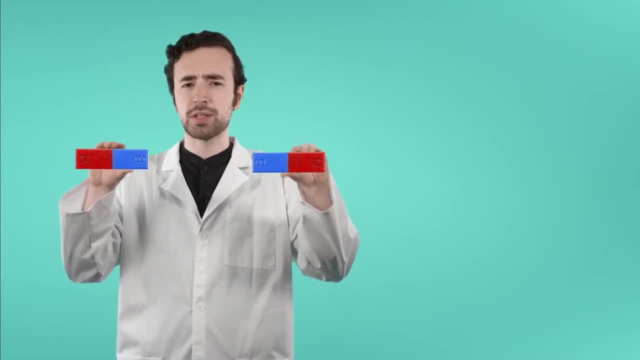 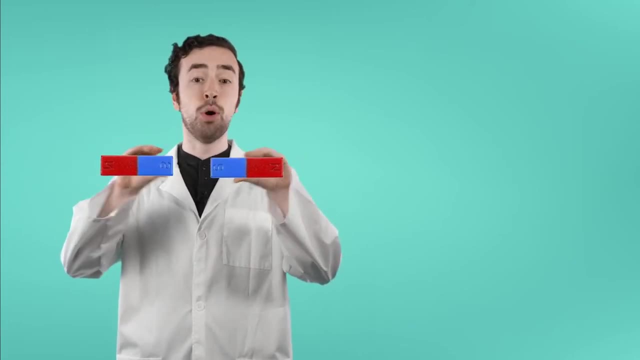 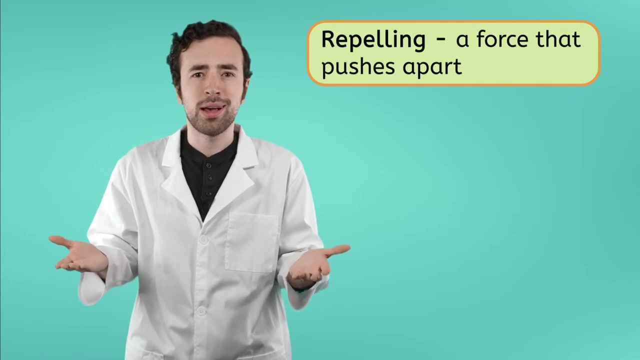 they just won't go. It feels like there's an invisible force field between them. Well, here, the force of magnetism is actually pushing these magnets apart or repelling them. So how does any of this actually work? How can there be a force that we can't see? 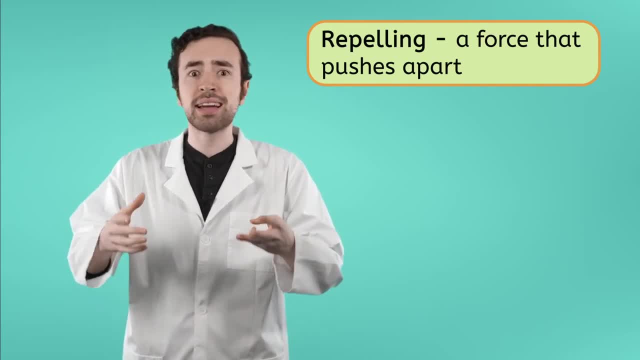 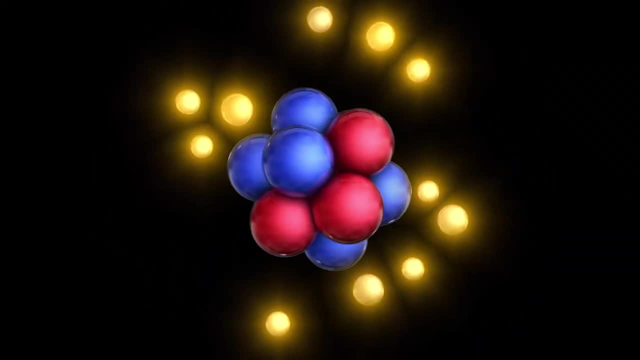 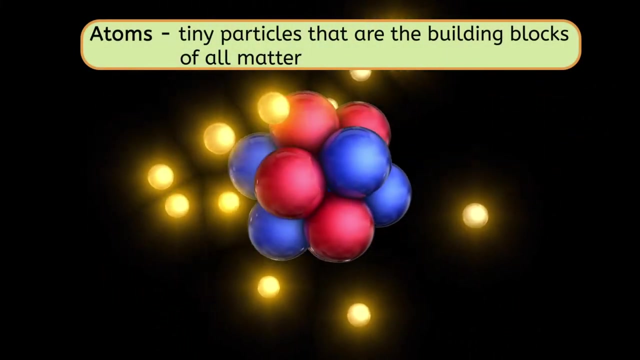 that can act on objects without even touching them and can both push and pull. To understand magnetism, we have to look all the way down at the atomic level. As we know, all matter is made of atoms, those tiny particles that are the building blocks of everything in our universe. 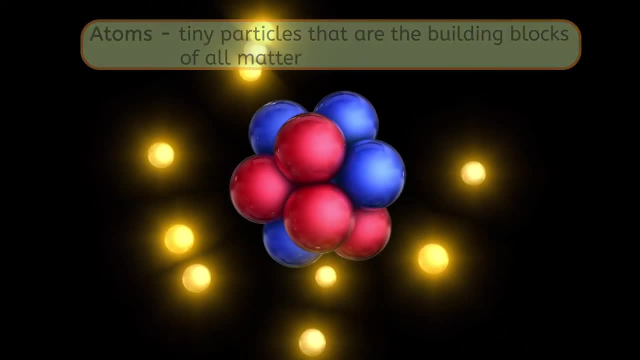 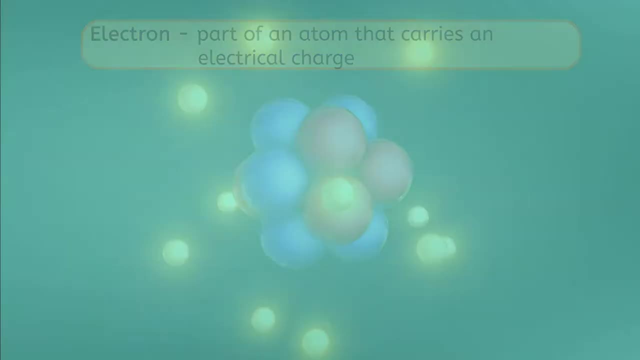 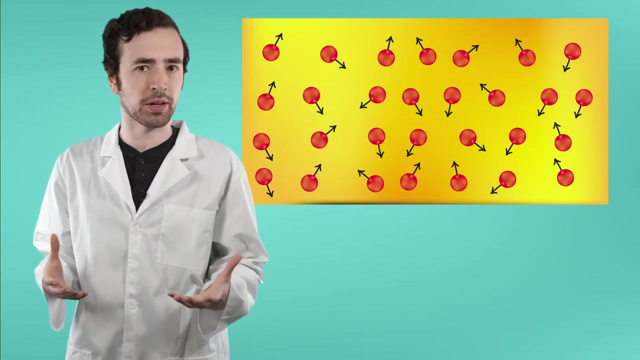 Atoms themselves are made up of even smaller particles, like electrons, which carry an electric charge. In most materials, these electrons are spinning around the outside of the atom in all different directions. However, in magnets, the electrons are all spinning in the same direction. 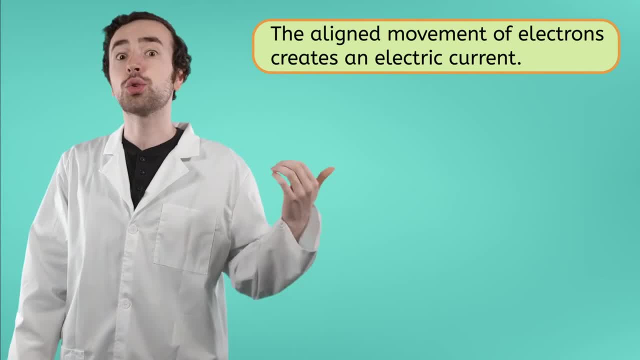 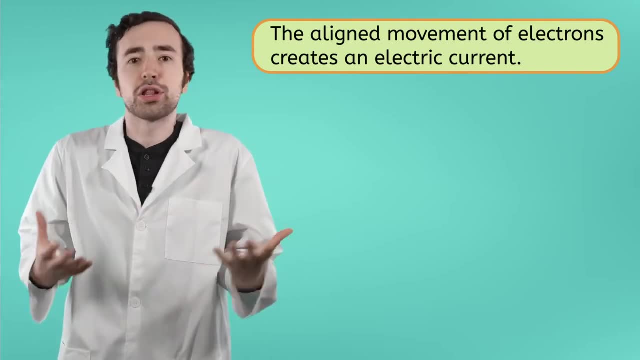 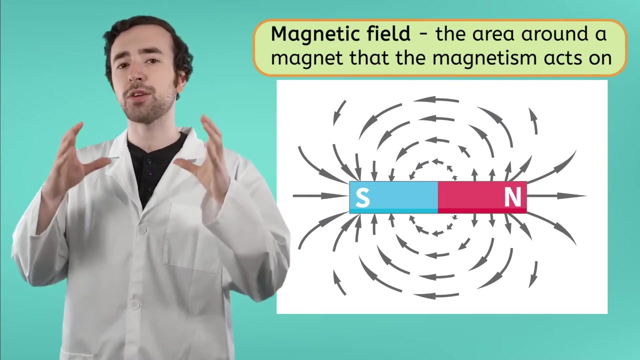 This aligned spinning of the electrons creates an electric current, and that's what causes the force of magnetism. This aligned electron spinning also creates a magnetic field. That's the area around a magnet where the magnet's force can act on. That's how magnets can attract and repel things without. 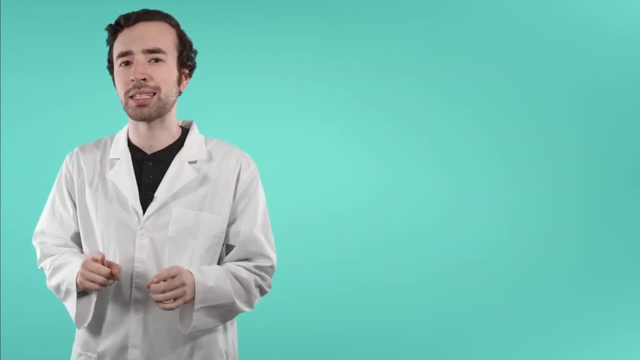 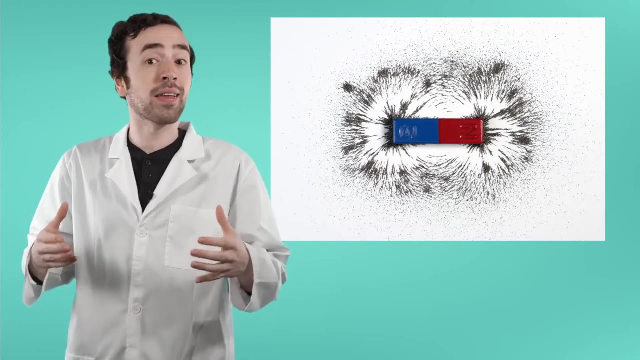 even having to touch them. You can actually visualize a magnetic field by placing lots of little bits of iron filings on a surface around a magnet. The iron filings are magnetic, so they'll align to the magnetic field, making it visible. It's pretty cool right. 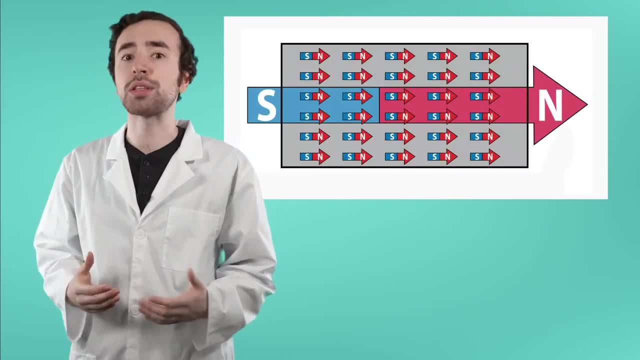 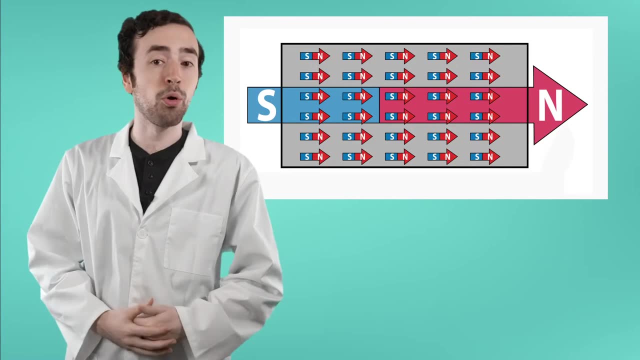 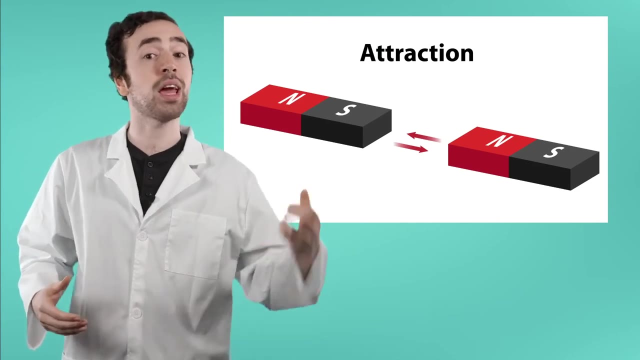 So since all these electrons are facing the same direction, there is a pretty clear front end and back end to a magnet. We call these ends the north pole and the south pole. right, When it comes to magnets, opposites attract. So if you try to match a north pole to a south pole of another magnet, 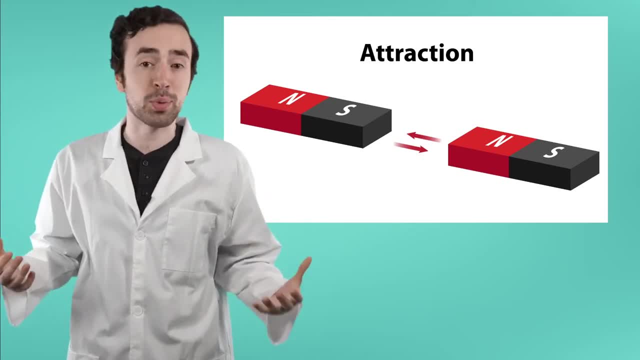 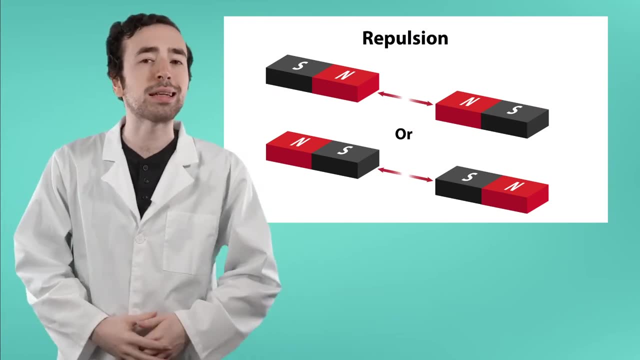 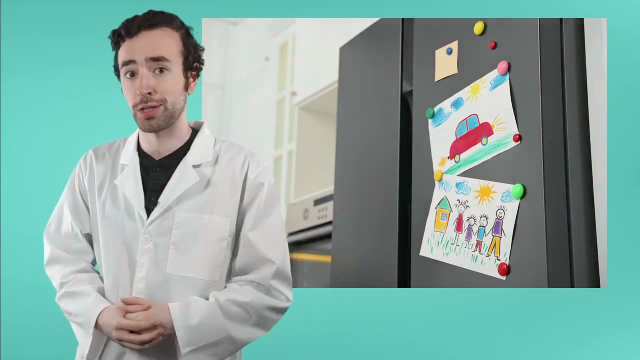 then they will attract. However, if you try to put together two north poles or two south poles, then the magnets will repel. Once we understand how magnets work, we can use them for all sorts of useful things Besides just displaying your hard work on the fridge. 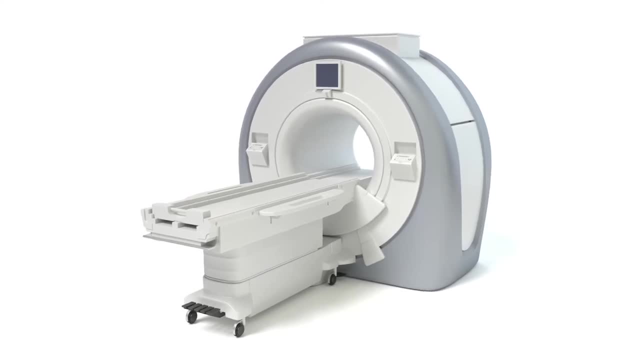 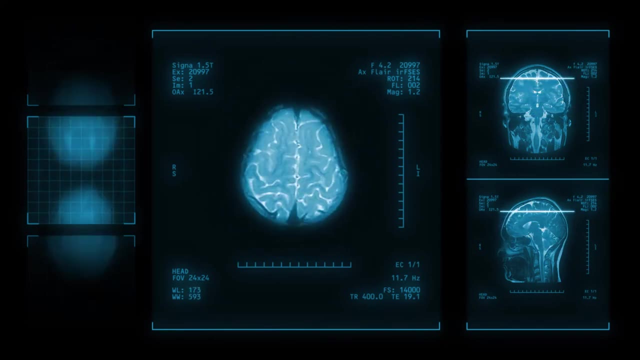 For example, magnets are used in MRI scanners to create an image of the inside of a person's body, which doctors can use to help people when they're sick. Electromagnets which are super strong because an extra electrical charge is run through them. 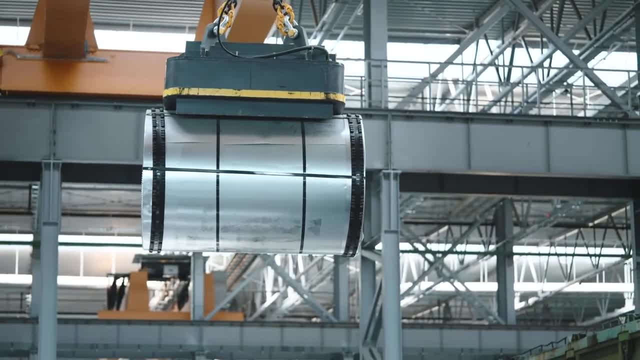 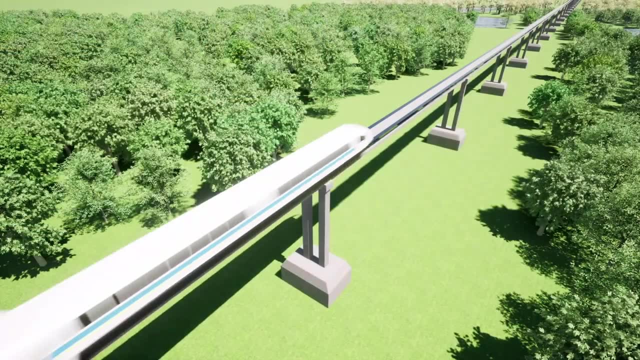 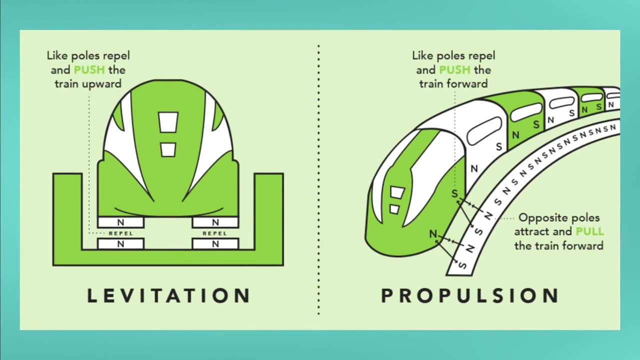 are used for big jobs like construction. One of the newest ways to use magnets is with maglev trains, which use the attractive and repulsive forces of magnets to hover a train above the track, eliminating the force of friction that's normally on train wheels. 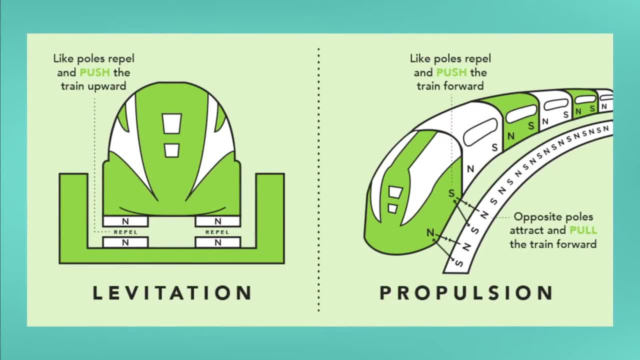 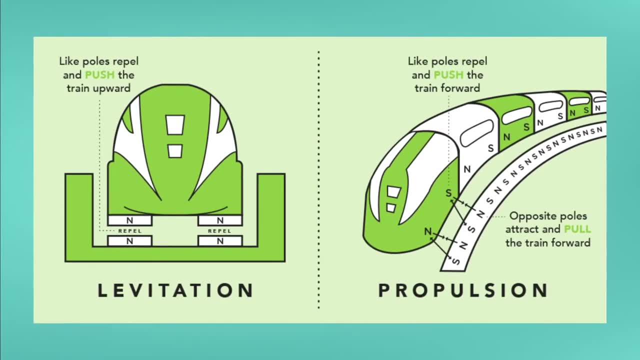 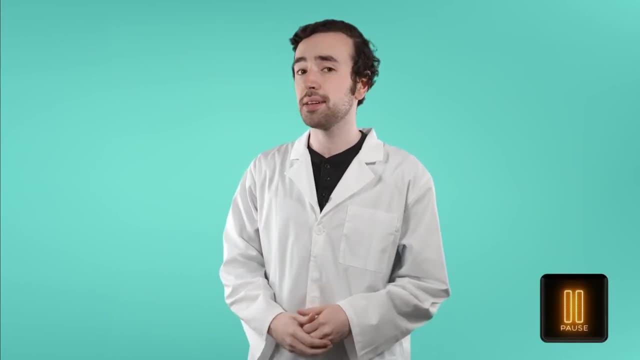 Using only the force of magnetism, maglev trains can move much faster than a normal train, up to 375 miles per hour. Can you think of some other places where we use magnets? Pause the video here and write down your ideas in your guided notes. 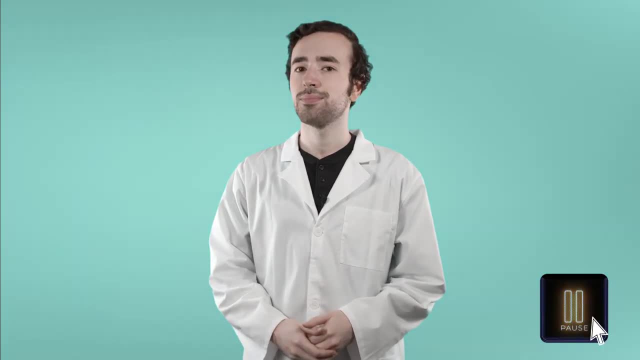 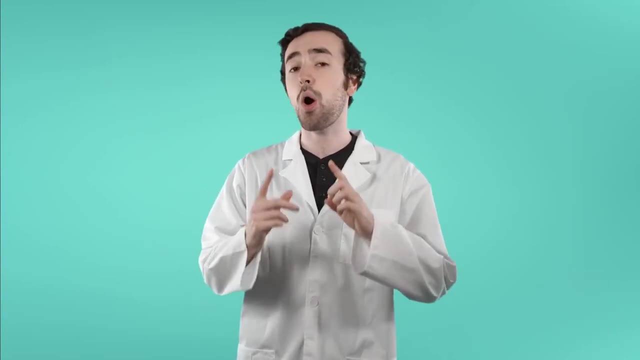 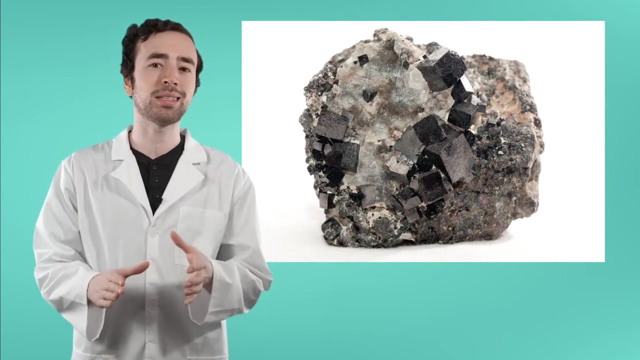 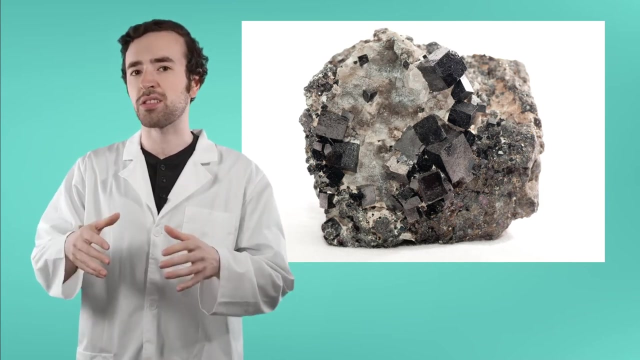 Magnet Tracking. Now, most of the magnets that we use in our day-to-day lives are man-made, But there are magnets in nature too. Take lodestones, for instance. These are magnetized pieces of the mineral magnetite. It's believed that they get magnetized by the electric current from lightning strikes. 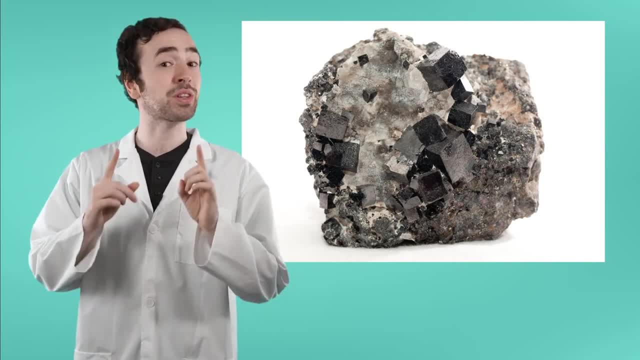 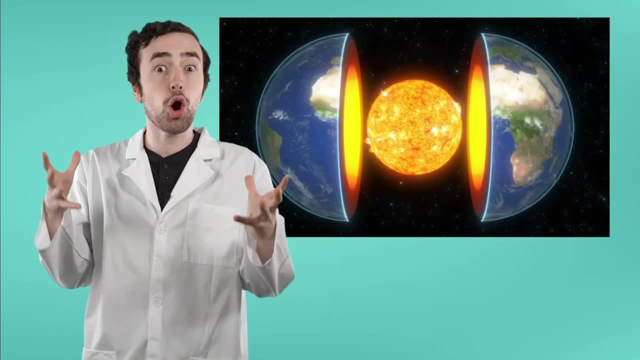 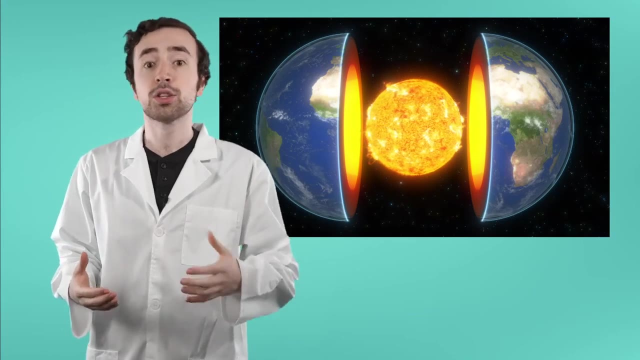 People used lodestones in ancient times as the first compasses. One of the biggest natural magnets out there is actually the Earth itself. The core of the Earth is made up of molten iron and nickel, so the movement of those liquid metals creates a magnetic field over the entire planet. 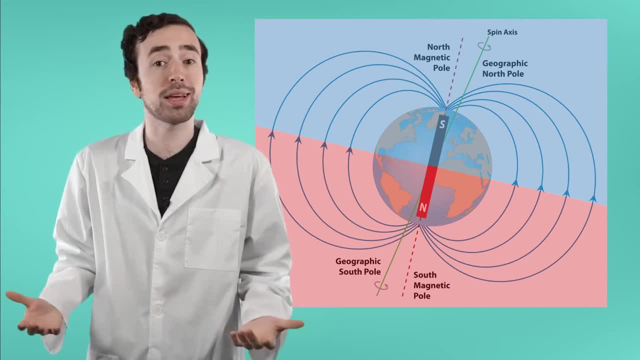 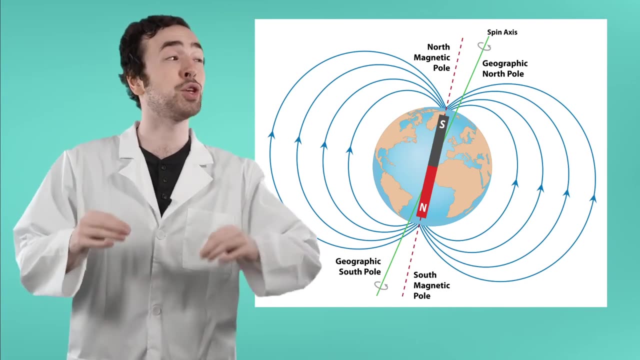 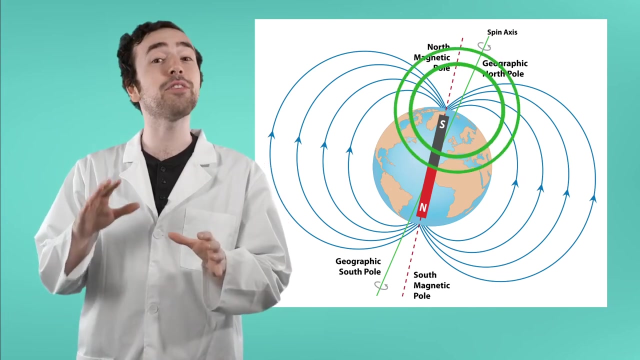 complete with its own North and South Pole, just like any other magnet. Now, Earth's magnetic North and South Pole aren't exactly where its geographic North and South Pole are, but they're actually pretty close. Earth's magnetic North Pole is about 500 miles away from THE North Pole. 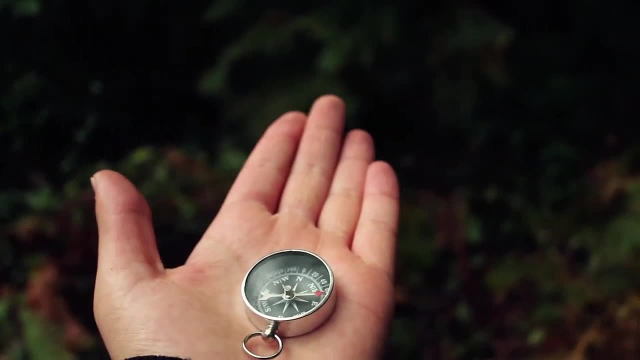 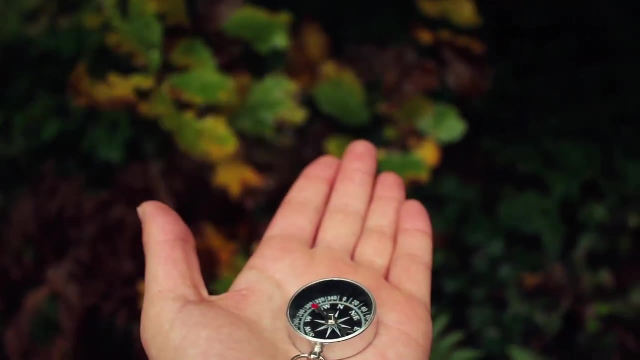 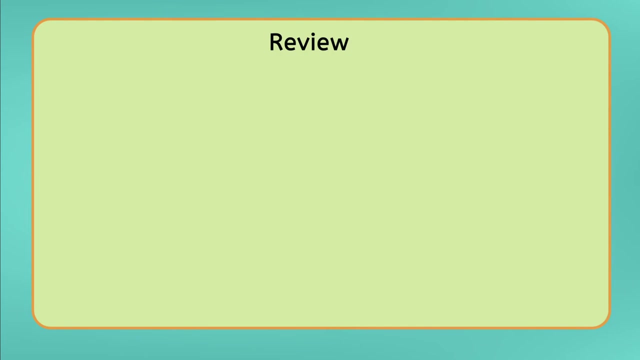 The Earth's magnetic field is the reason why compasses are so useful for navigation. They point travelers north, because the magnets in a compass are pulled to Earth's magnetic North Pole. Pretty cool. Let's review everything we've learned today about magnets. Magnetism is the force exerted by the 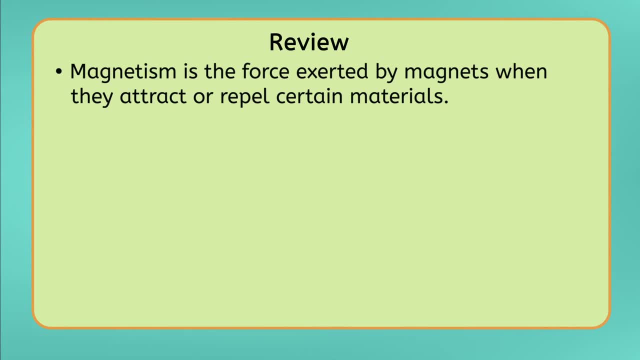 Magnets, when they attract, pull or repel, push certain materials. Iron, cobalt and nickel are the most magnetic materials. Magnetism is caused by the flow of aligned electrons. Opposite poles of a magnet attract and like poles repel. 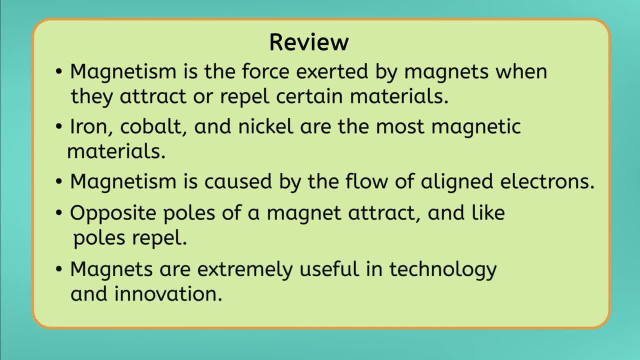 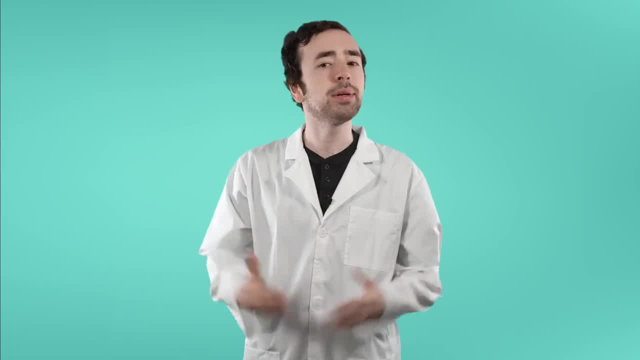 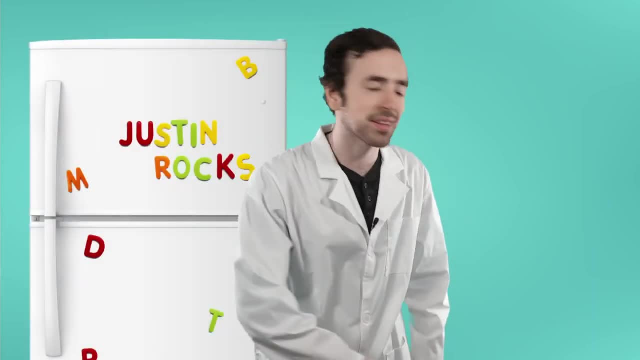 And magnets are extremely useful in technology and innovation. To learn more about magnets and magnetism, be sure to check out the activities and practice questions for this lesson. Now, if you'll excuse me, with all the magnets in the world, I gotta start spreading my message. 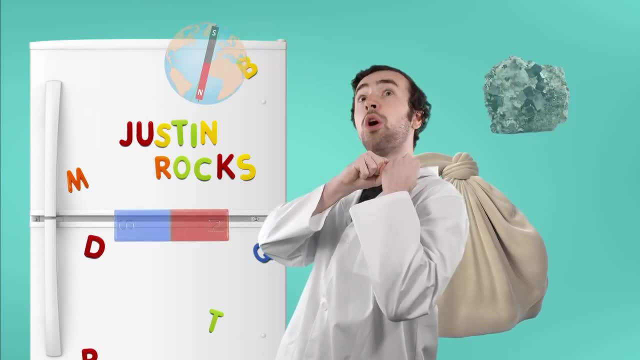 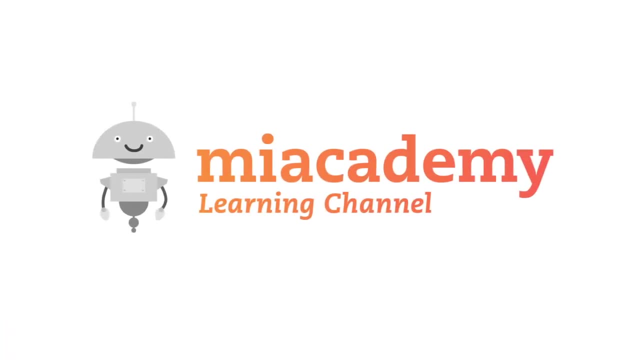 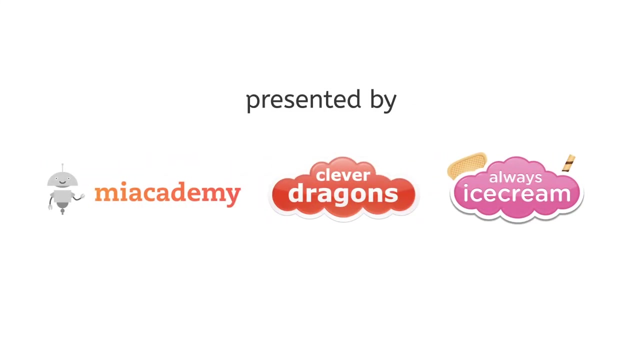